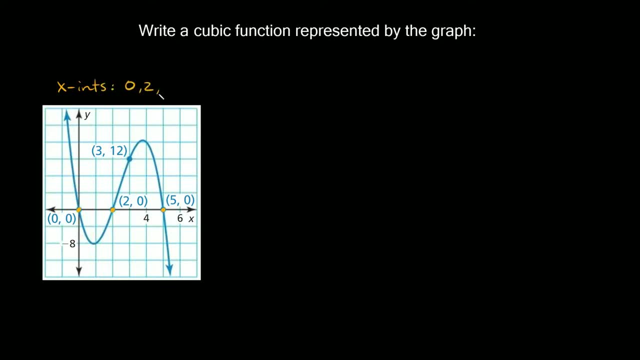 So we have them at zero, two and five. Okay so, since we know the x-intercepts, we can use the intercept form of a function to write out our function. So it's going to be: f of x is equal to a times x minus p, times x minus q, times x minus r. Okay so, since we have three x-intercepts over, 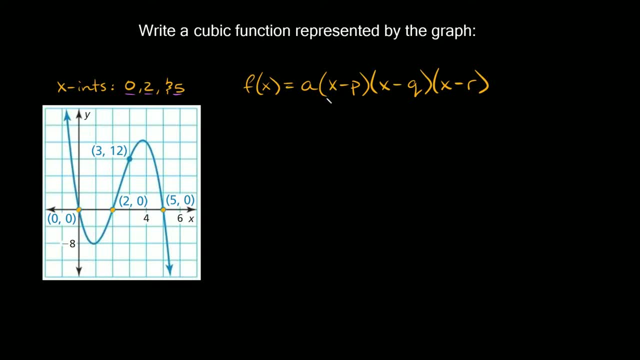 here. that's why we need to write out the x-intercepts. So let's write out the x-intercepts. So we need three sets of parentheses over here, So x minus p, x minus q and x minus r. Okay, and that's normally going to be the case with cubic functions, You're normally going to have three. 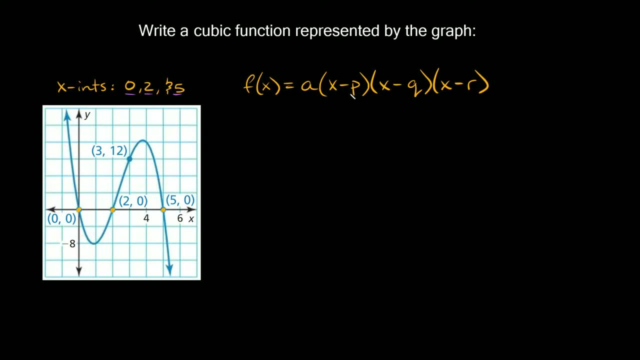 x-intercepts. So three sets of parentheses, Okay, and just to break this down again, this a right here is just a coefficient. and then p, q and r are your x-intercepts right. So that's why, again, since we have three x-intercepts, that's why we need our three sets of parentheses, right here. 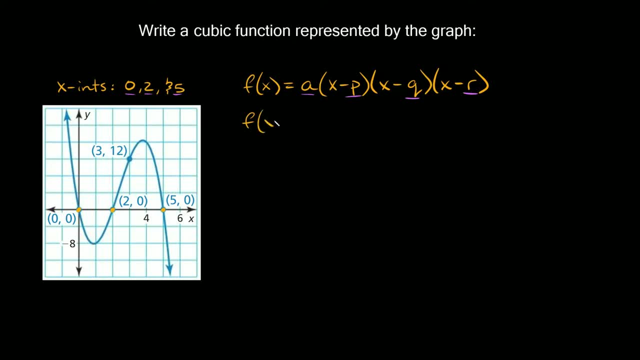 Okay, so let's start filling this out. So we're going to need to have f of x is equal to a, and then, in this first set of parentheses, we're going to put our first x-intercept, which is zero. So we're going to write x minus zero, and then here we're going to have x. 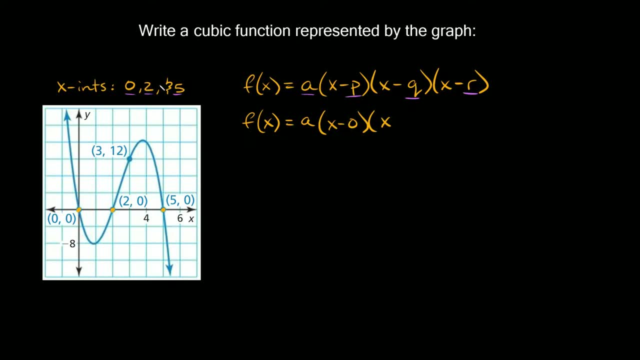 and then here we have a positive two. Now, when you plug in your x-intercepts into your parentheses over here, you have to change the sign. Okay, so since we have a positive two here, we have to write it as a negative two or minus two over here. Okay, and then same thing with the last one here. 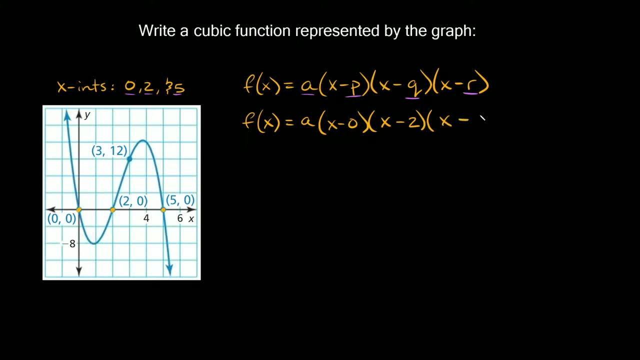 We have a positive five, so here we have to write it as x minus five. Okay, the last thing we have to solve for here is a, and the way you solve for a is by using, basically the fourth point that we're given here. that is not an x-intercept, and you plug that in to your function. Okay, so three we're. 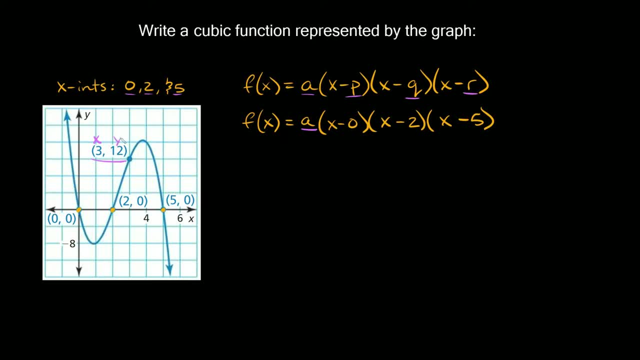 going to plug in for x and twelve we're going to plug in for y, or in other words, f of x. So here this is going to be equal to twelve, right? so we're going to say twelve is equal to twelve, equal to a, and then, in parentheses, x minus 0. but again we're going to plug in a 3 for our x's. so 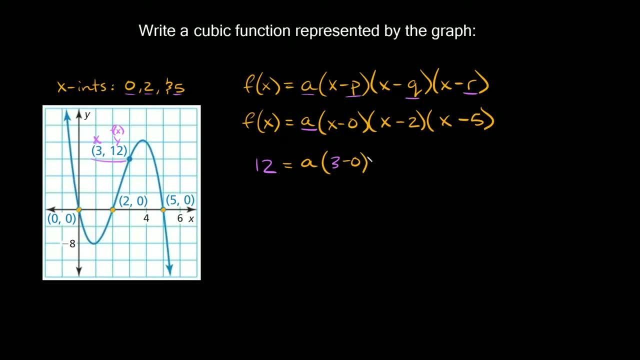 we're going to have 3 minus 0 times 3 minus 2 times 3 minus 5.. So then here we have: 12 is equal to a, and then 3 minus 0 is just 3.. 3 minus 2 is equal to 1, and 3 minus 5 is equal to negative 2.. 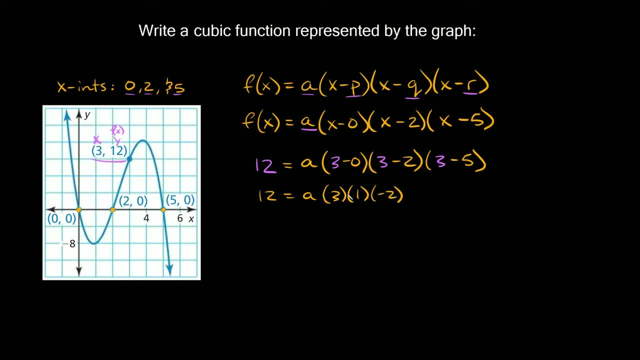 All right, 3 times 1 times negative, 2 is equal to negative 6.. So this is- I'll just write it over here- we have: 12 is equal to a times negative 6, and then to solve for a, we'll divide both sides. 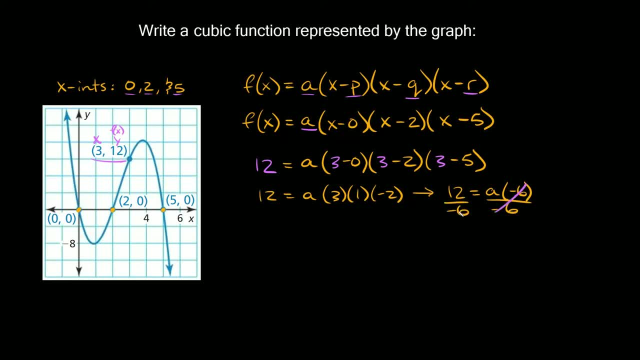 by negative 6.. All right, those cancel out. so 12 divided by negative 6 is equal to negative 2. so we get: negative 2 is equal to a All right. so that's where we're going to plug in for our a right here. Okay, so I'm just going to bring this down right here. 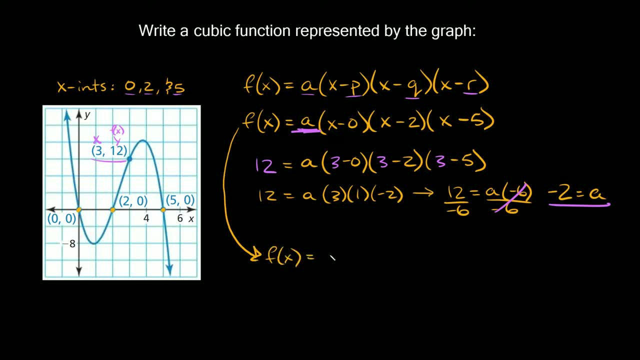 So this is going to be: f of x is equal to negative 2, and then here we have x minus 0. So this we can really just write as x. Okay, because when you add or subtract 0, it doesn't change the value of x. 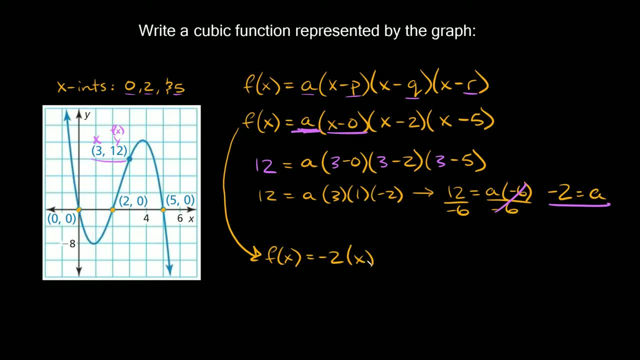 right. So whenever you have an x minus 0, you can simply write it as x. Okay, and then here we have x minus 2 and x minus 5, right, So x minus 2 times x minus 5.. Okay, now, multiplying all this crap together, negative 2 times x, that's equal to negative 2x. and then here: 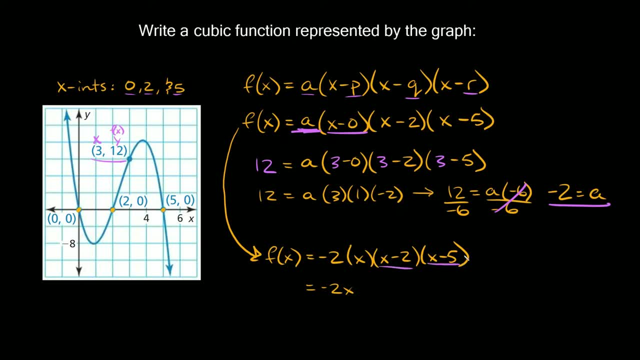 we have a binomial right: x minus 2 times x minus 5.. So in order to multiply two binomials together, you just need to FOIL. So if you don't remember what that is, I'll link a video to that in the 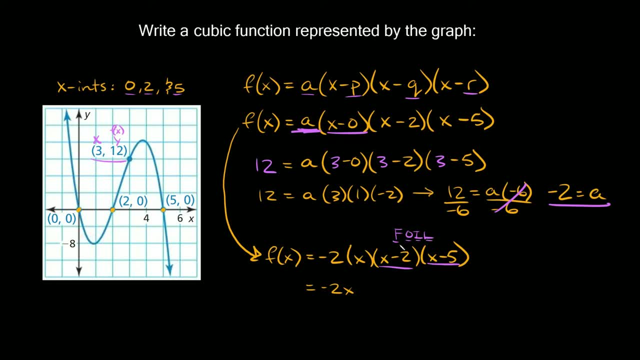 card above. but this stands for first, outer, inner, last. So that's the order that you multiply the binomials in: Okay, so you're going to go first, then outer, then inner and then last. So you're going to go first, then outer, then last. Okay, so multiplying that all together we're going to get